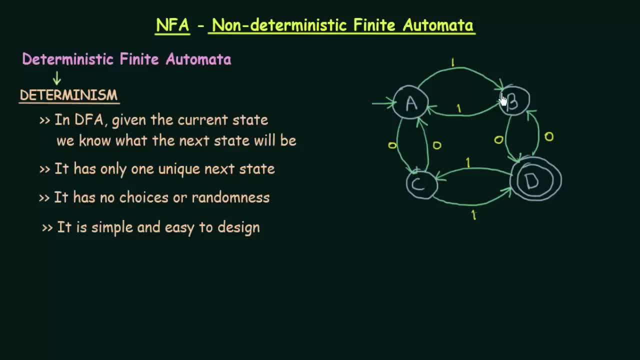 So, given the current state, we are sure about what is the next state on getting particular inputs. Alright, And then it has only one unique next state. So suppose again, I am seeing for state A, I am in state A and if I get input 1, it goes only to state B and not to any other states. 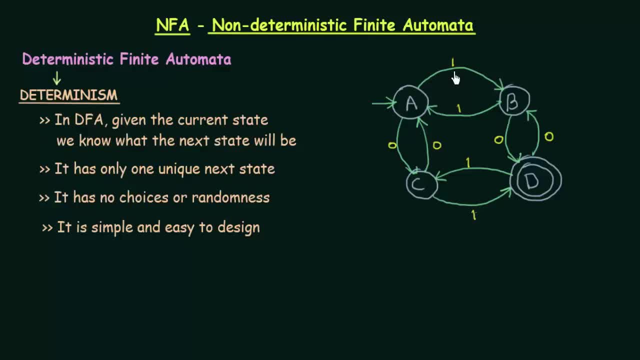 Right, So it has a unique next state. On getting input 1, it goes to the next state, that is B. It does not go to any other state. So, on getting certain inputs, each state has a unique next state. 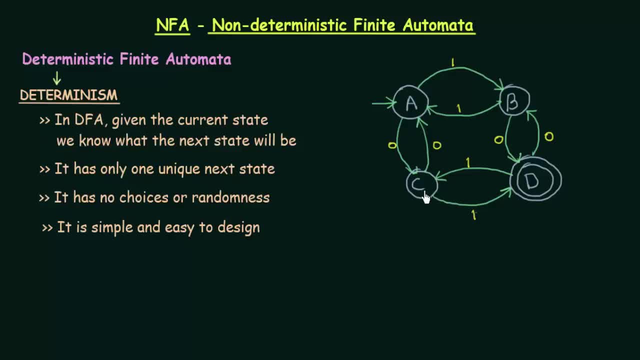 Right. So if I Take for state C, for example, If I get input 0, it goes to state A and only to state A. On getting input 0, it does not go to any other state other than state A. 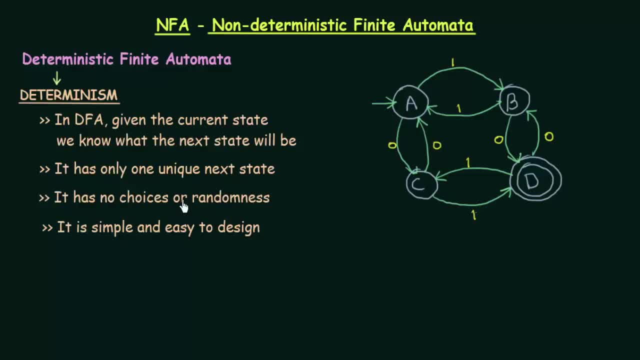 So it has a unique next state And it has no choices or randomness Right. Suppose I am in state A and I get input 1, it has no other choice than to go to state B. It does not go to any other choice other than state B. 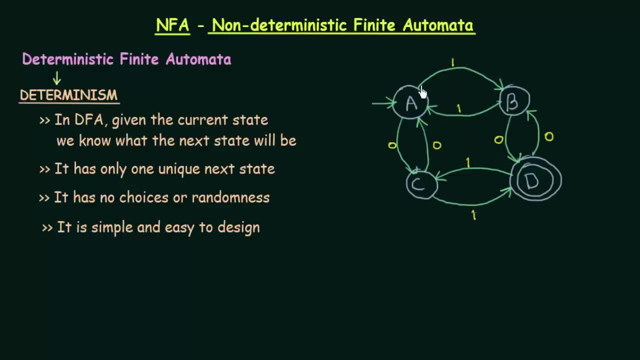 There are no other choices that it has to make. It is sure and it knows that it has to go to. It has to go to state B And it is simple and easy to design. Why is it simple and easy to design? Because we know that, on getting certain inputs, we know to which state we have to send it. 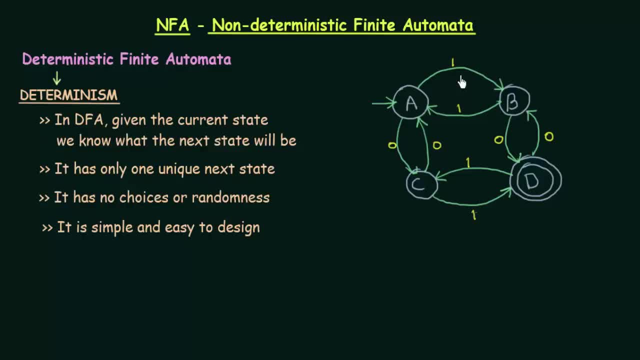 So we just have to design it showing the transition from one state to another on getting certain inputs. So that was about deterministic finite automata And that explained the determinism to us. Now, what is non-deterministic finite automata? 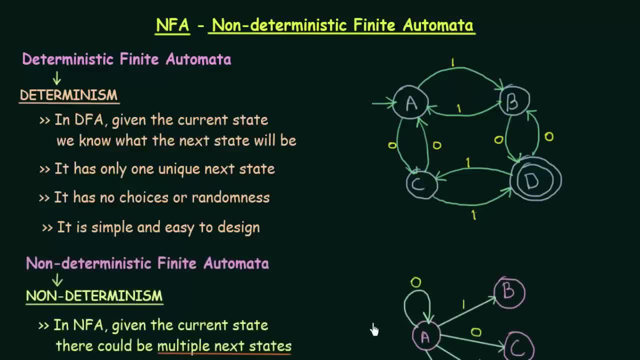 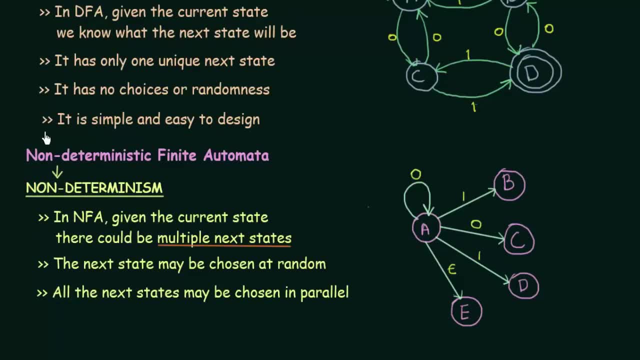 Okay, So non-deterministic finite automata it comes from the word non-determinism, So it comes from the word non-determinism, And what does this mean? So here I have a diagram of NFA, which is non-deterministic finite automata. 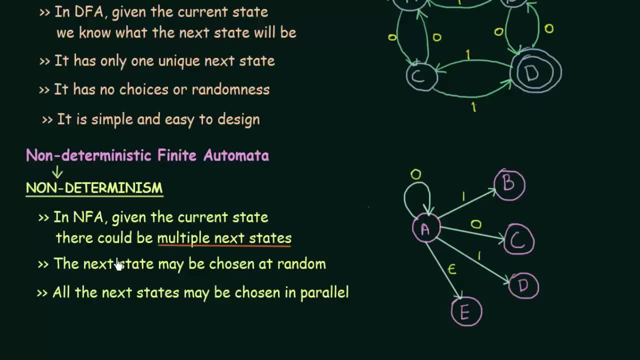 So in NFA, given the current state, there could be multiple next states. We know that in DFA, given one state, there is only one unique next state. But in NFA or deterministic finite automata, as I have shown here, 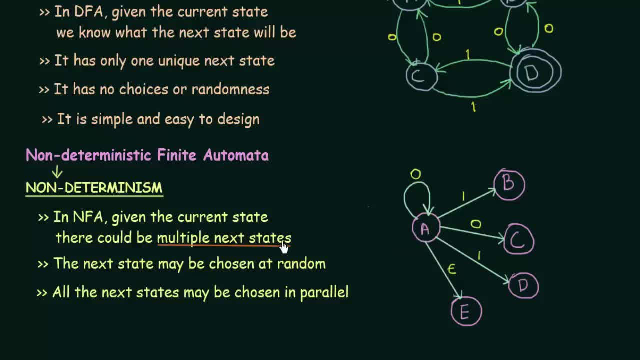 given a current state, there could be multiple next states. Now look at this. We have a state A here And A on getting input 0, let's see how it behaves. A on getting input 0, it could stay either in A itself or it could even go to state C. 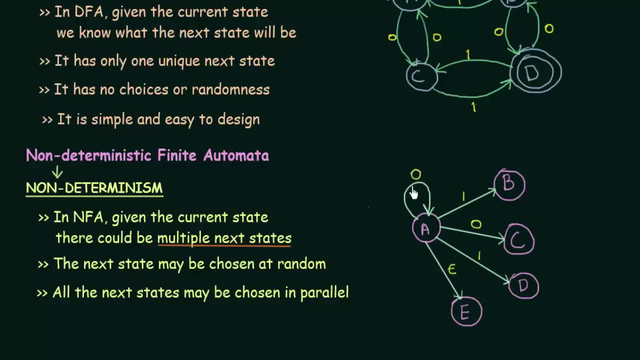 It can have multiple next states. On getting input 0, it could either stay in A itself or it could even go to state C. And let's see what happens on getting input 1.. On getting input 1, A could either go to B or A could also go to D. 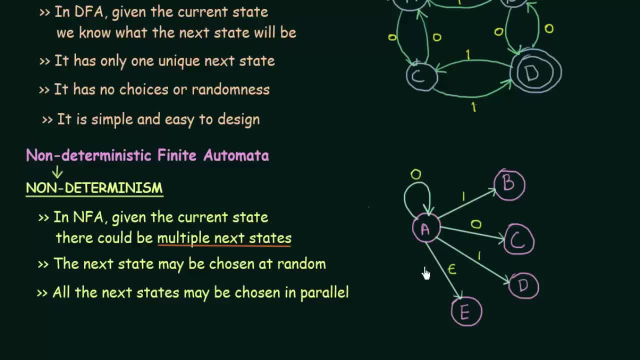 So it has multiple next states. Now the question is, how do you choose to which state it goes on getting a certain input, Because it has multiple next states. So it says here that the next state may be chosen at random. 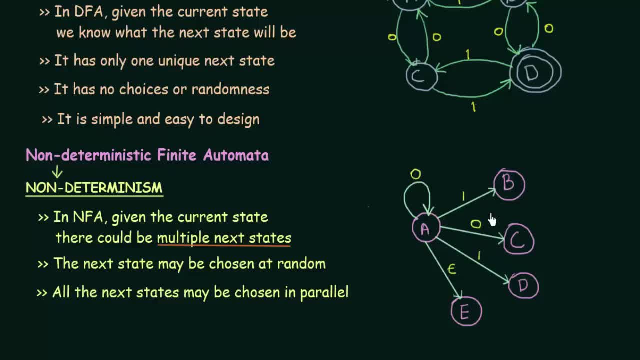 We may choose the next state at random. Just randomly you can choose it, Or all the next states may be chosen in parallel. You can either choose the next state in random or you can choose all the next states in parallel. That means you could simultaneously choose all the next states for a particular input. 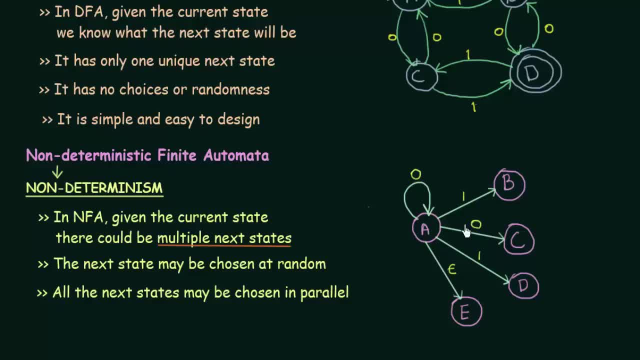 So that is about non-deterministic finite automata. And here you see something different which we have not seen in DFA, That is an edge that is labeled by epsilon. So what is this epsilon? I have already taught in the previous lectures that epsilon actually means the empty string. 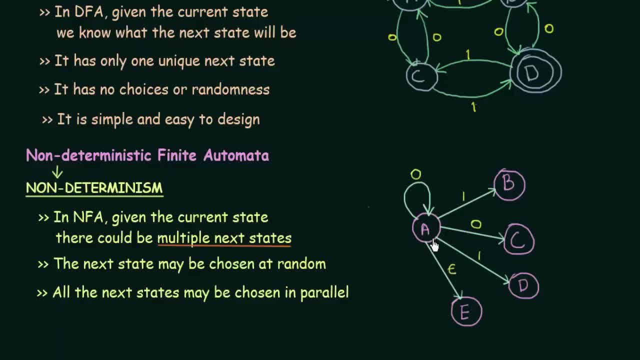 So this means that this state could also accept an empty string or an empty input And on taking that empty input it can go to another state, which I call state E. So this concept of epsilon: it comes only in non-deterministic finite automata. 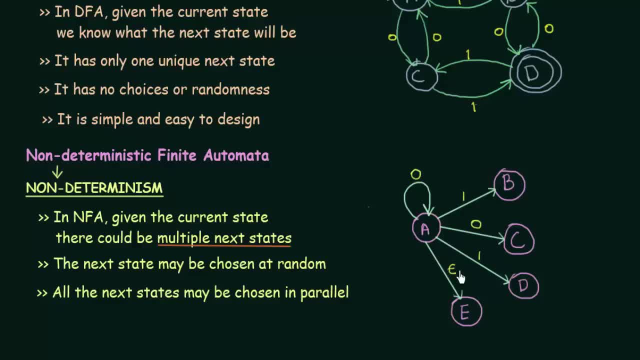 It is not there in our DFA. So if you see an epsilon, or if you see that a state is empty, if you see that a state is going to multiple states on getting the same input, then you should understand that it is a non-deterministic, finite automata. 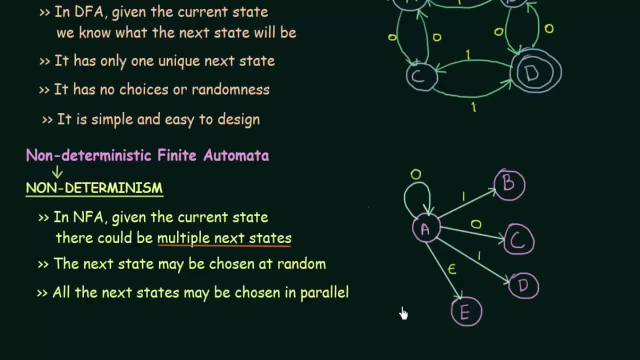 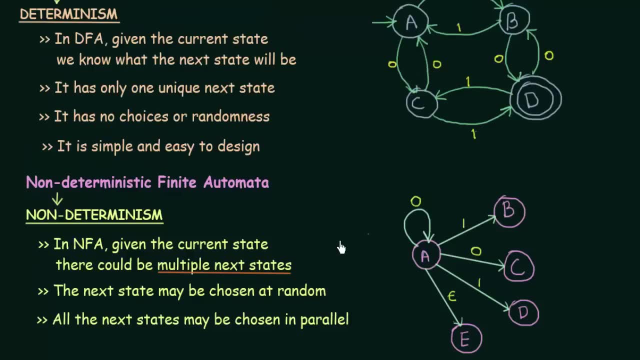 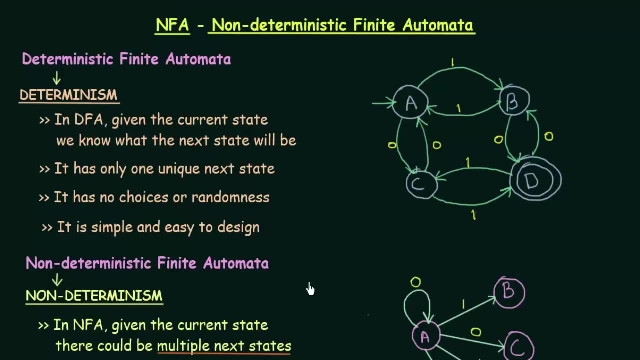 So when we take more examples in the next lectures it will become more clear to you. So I hope this made the concept of non-deterministic finite automata And you could also see the difference between deterministic finite automata and non-deterministic finite automata.